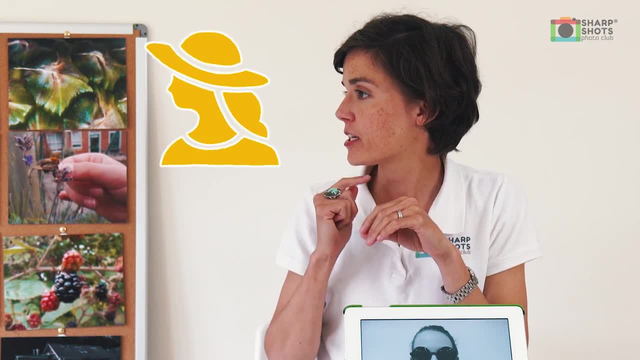 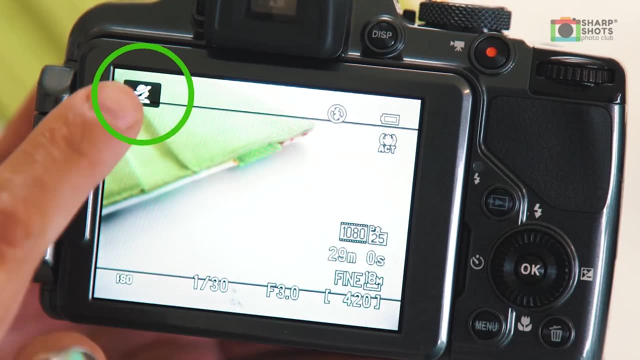 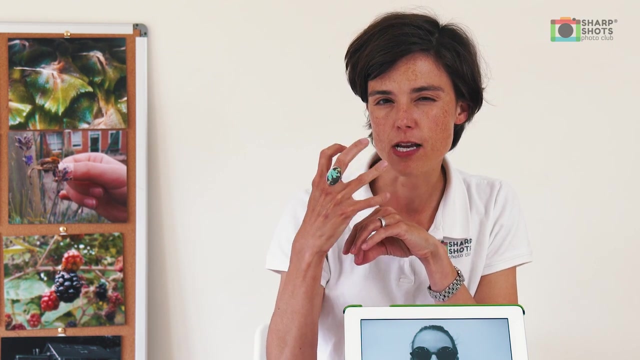 And this will look like the side view of a person. Generally, usually it's a lady and quite often it's on the top mode option on the camera or in the scene settings for you to choose. And by choosing the setting you have the ability to blur the background just a little bit and make sure that your subject, the person, is nice and sharp in the picture. 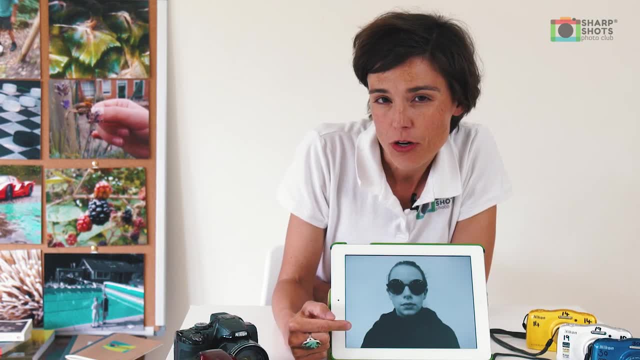 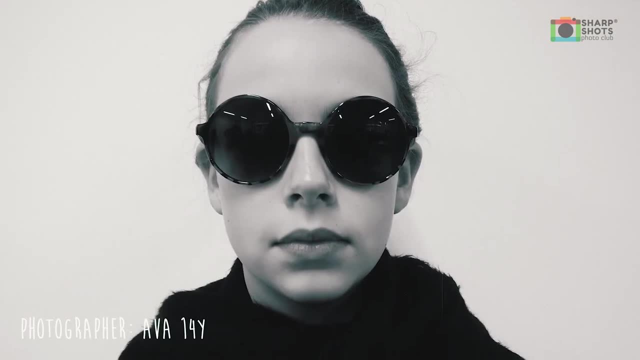 Sit down. If you have a look at this photograph here. your portraits don't always have to be in color. You can try switching it on to black and white, which can work quite well. The photographer here has photographed someone that perhaps is into fashion. 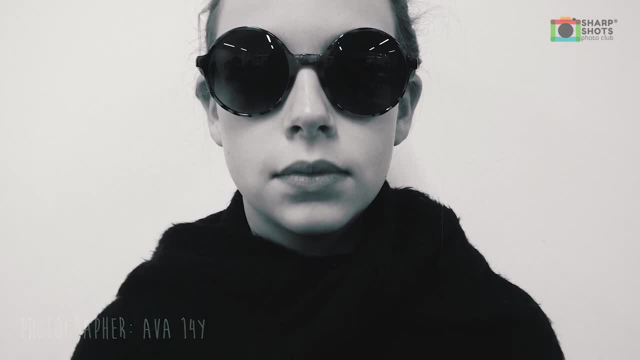 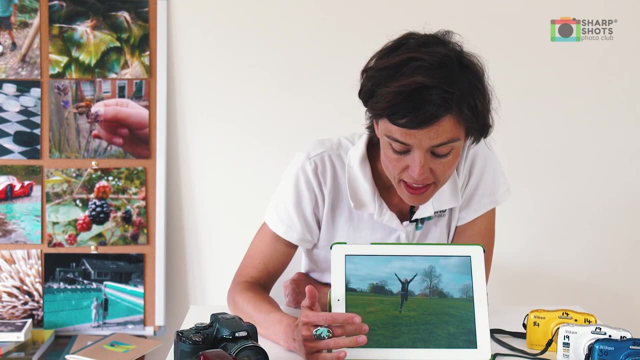 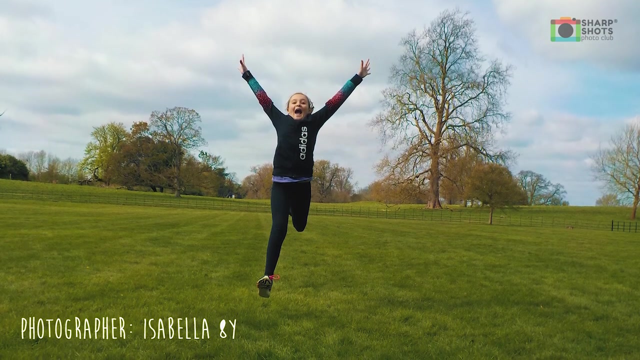 So she's got big sunglasses on, She's got some lovely lipstick and is looking quite serious. So perhaps that's her nature- She has a bit of a serious edge to her. The photographer here has captured their friend in the garden having a bit of a run jump and a laugh, it looks like, which is quite nice. 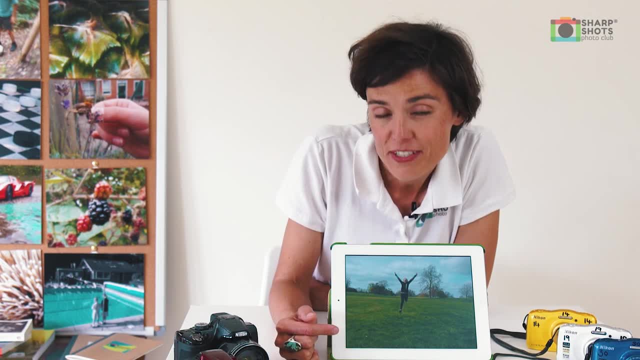 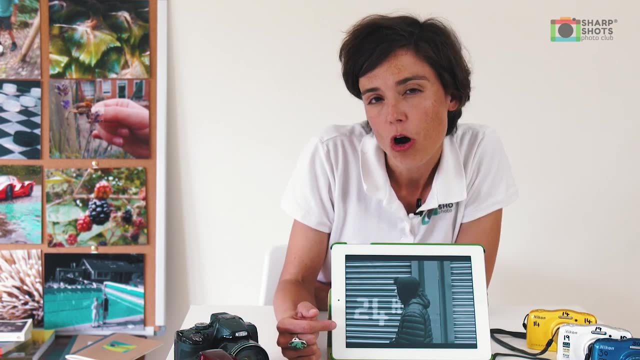 Really relaxed, Quite inspiring, And they're obviously both having fun doing it, which is the main thing This image here shows you don't always have to be looking at the camera Quite often. I would suggest for my subject to look up down away. 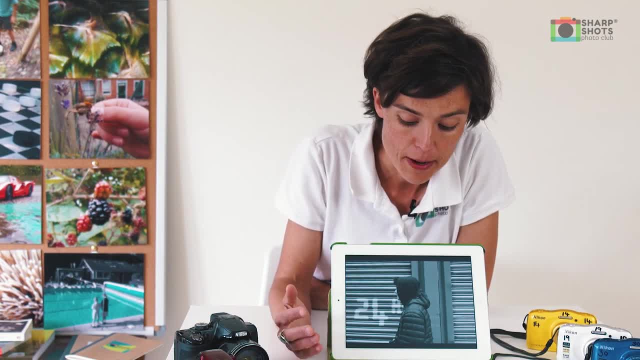 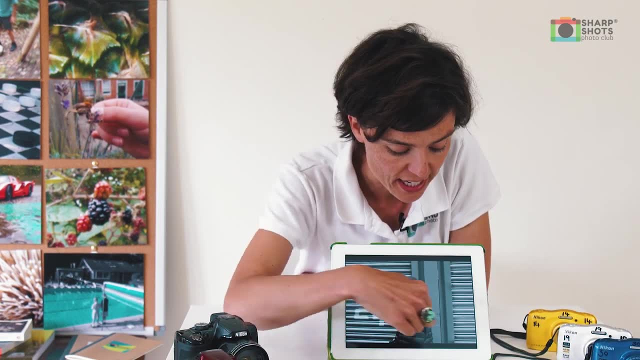 It gives the photograph a different feel. It can feel perhaps a bit more distant or you learn a little bit more about what they're wearing. You see a lot here. The lines work really well with the jacket in the background And you can tell they're in a bit of an urban setting. 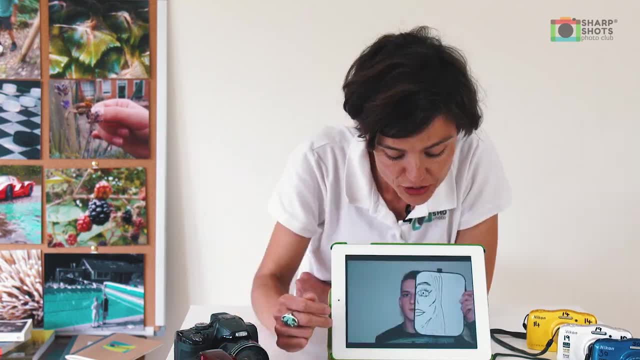 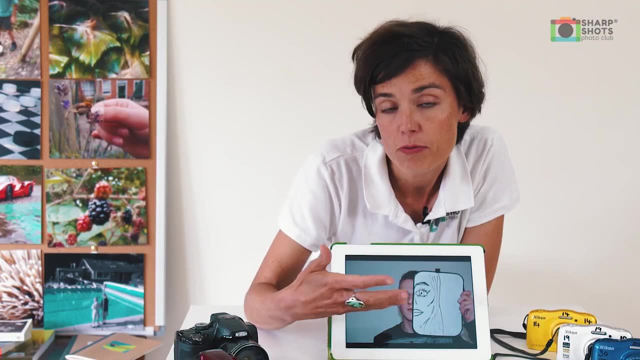 With the 24 going behind as well. If you look at this photograph here, the photographer has entered a prop into the picture, Which I think really works well, because we know that this chap likes to probably draw, And you can tell he's quite good at drawing as well. 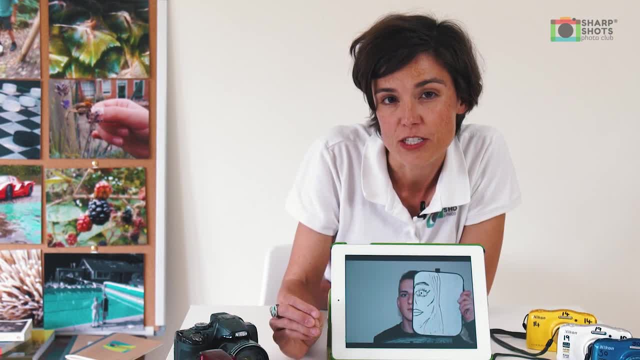 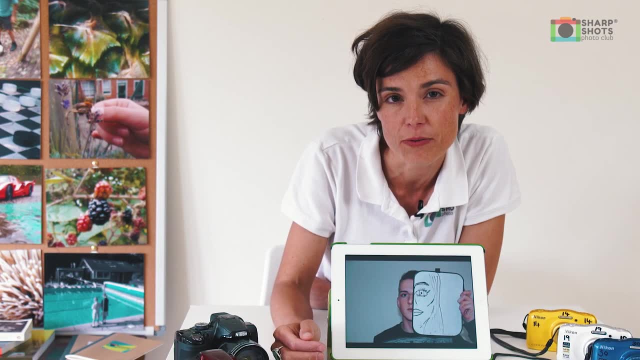 And it adds another layer onto the picture, which makes it a lot more interesting for us as viewers to look at too, And I really like how he's looking, and the drawing is looking at us too. The engagement works really well here. And the last photograph I wanted to show you was 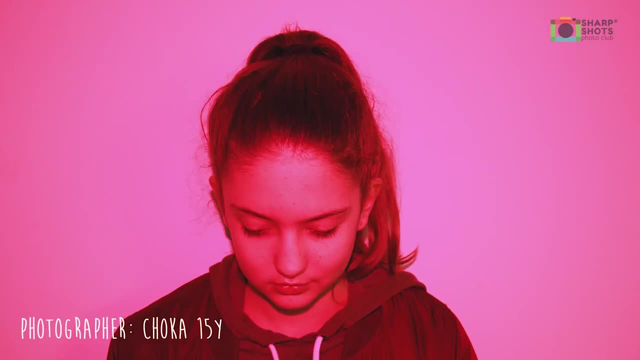 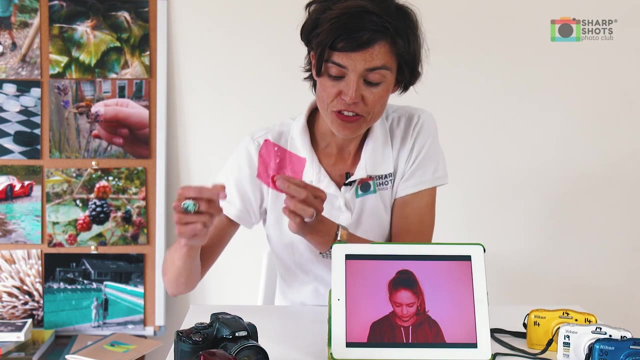 Was this image here that looks quite pink, And this is quite a fun way to take a photograph. You introduce a little gel onto the picture And this is taken from a quality street, which is quite fun. All you do is put it straight onto the flash, like that.